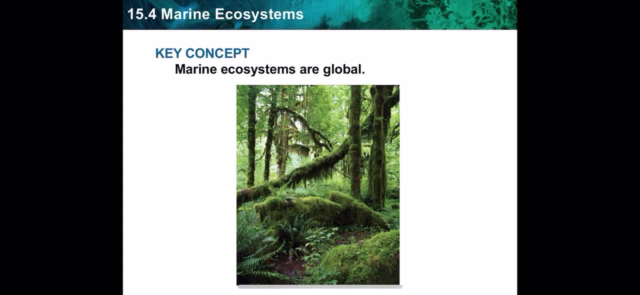 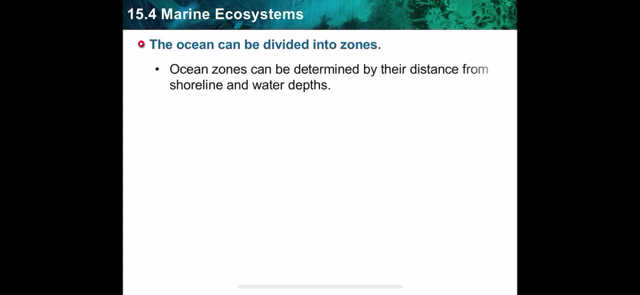 the difference between marine ecosystems and freshwater ecosystems, The difference in the salinity of water, Salty water, marine ecosystems, Freshwater, freshwater ecosystems. If I asked you where can I find marine ecosystems? so obviously you will tell me in ocean and seas, But actually, 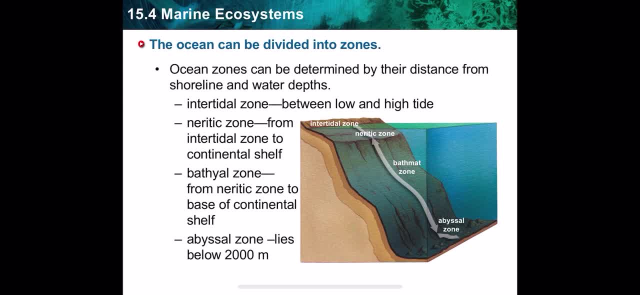 the ocean is the largest water body. so do you think the ocean consists of only one zone With homogenous climatic, with homogenous abiotic and biotic factors? same communities can live in all the areas of the ocean? Of course not. The ocean is divided into zones. 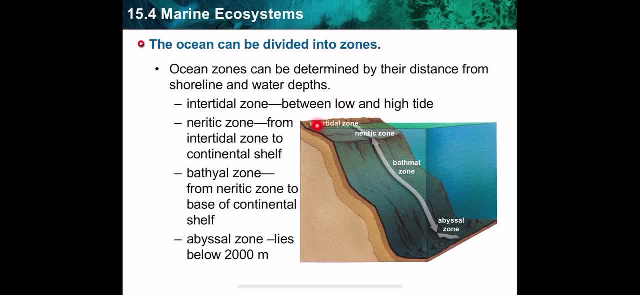 What are those zones? The first zone is the intertidal zone. From its name it's intertidal, so it's exposed to tide- high tide and low tide- From the end of the intertidal zone till the continental shelf, it's the neuritic zone. 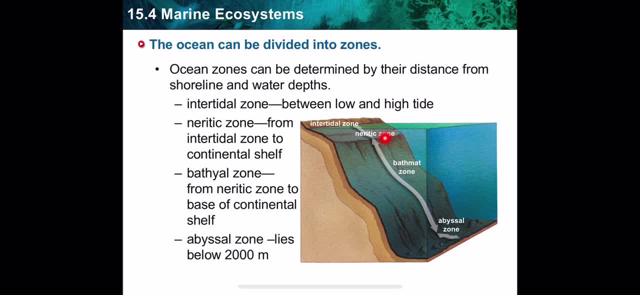 Enter tigal zone and neuritic zone. Both of them are in coastal oceans. After coastal oceans, open ocean- All this blue area is, and open ocean and Open oceans compose of two main zones, starting from the neuritic zone till the base of the continental shelf. it's the bathyal zone and thenumeric zone. 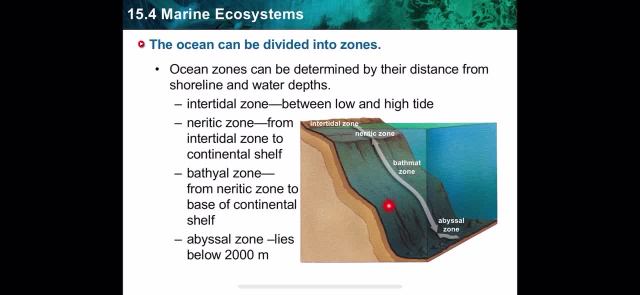 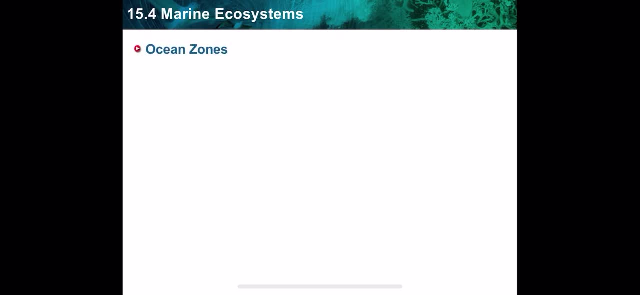 options. tell the views of the continental shelf. it's the back of the shell zone, but then they like zone after 2,000 meters till the ocean floor is the abyssal zone. enter tidal zone is the area that is exposed to high and low tide. look, here is the. 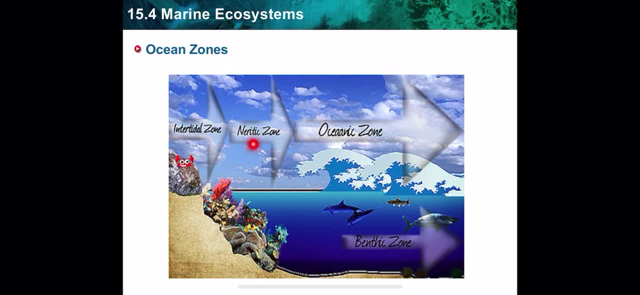 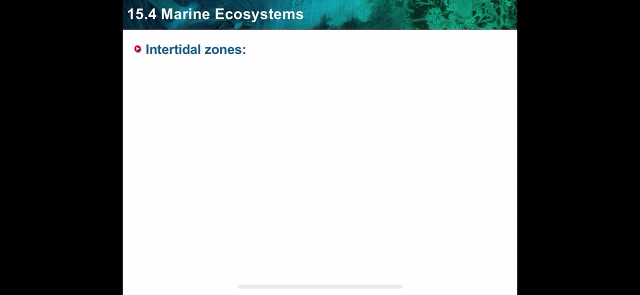 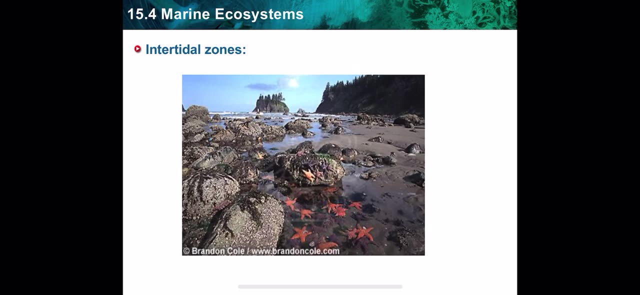 intertidal zone and the coast narrative zone, then oceanic zone, which contain bath yell and abyssal which is on, is it? it's the intertidal zone. how did you know? because some areas are exposed to air, other areas are covered with water, and even the areas that are covered with water, sometimes they are not covered. 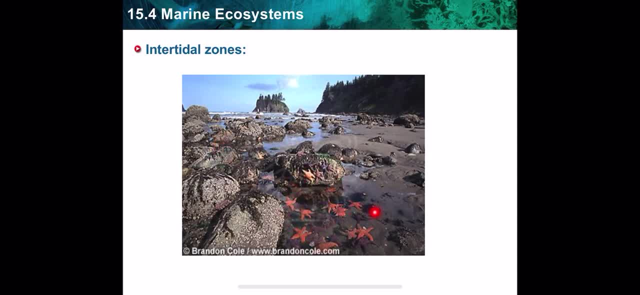 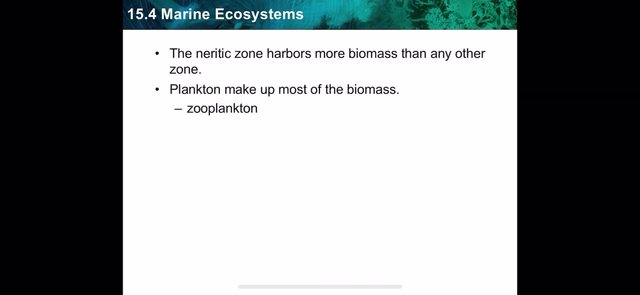 with water. so which abiotic factors are affecting organisms that are living there? number one: exposure to sunlight, exposure to air, exposure to wave action and, finally, change in salinity because of the difference water, the different water levels. as I told you, after intertidal zone, there is narrated zone. narrated zone is the zone which is characterized. 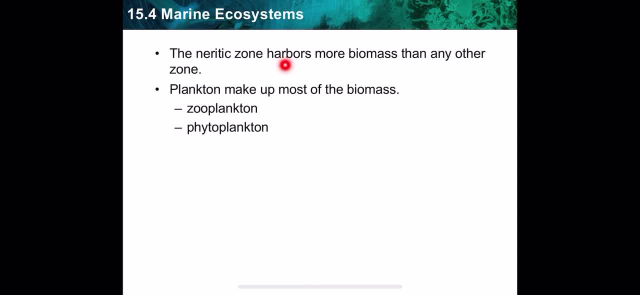 by the highest biodiversity in among ocean zones. so the narrated zone harbors more biomass than any other zone. why? because the learn epic Zone contains plankton's, what our plankton's, plankton's, our organisms, that make up most of the biomass. so most of the 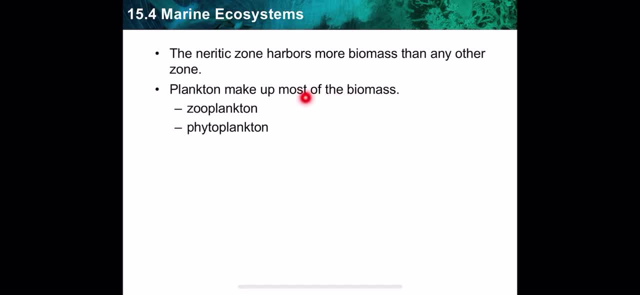 biomass. most of the biomass is from plankton's planks. are producers or consumers? actually, there are two types of plankton: zooplankton and phytoplankton. zooplankton, our zooplankton are zooplankton, are zooplankton box plants. those zooplankton is the species called. zooplankton are the species of the plant, plant which is the main source of lığımız zooplankton and phytoplankton. so as long as the plant mass, the plant mass works, this is the zooplankton of zooplankton are plants, and so on. it is heterogeneous zones, so we have pr 꽃 gera, Edit хx пох whitening. 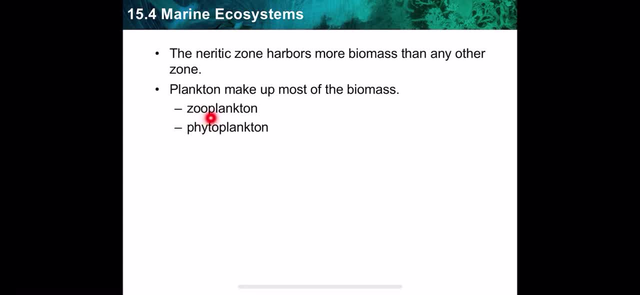 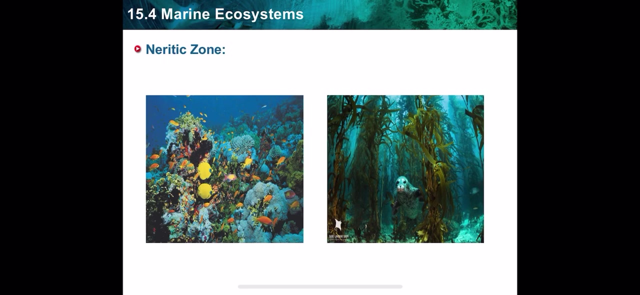 zooplankton, phytoplankton, phytoplankton- zoo, so tiny animals, so zooplanktons are consumers, phytoplanktons from phyto, from photosynthesis, so phytoplanktons are algae and photosynthetic bacteria and phytoplanktons are producers. the enritic zone also. in the enritic zone we 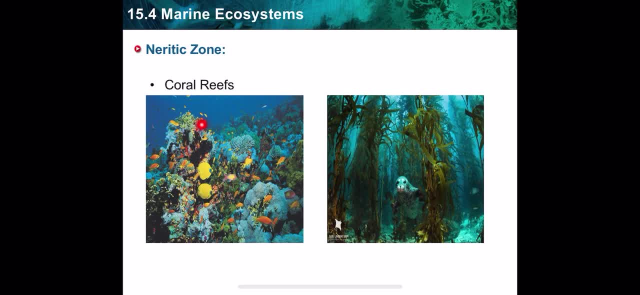 can find coral reefs? coral reefs- what are coral reefs? animals that live in a mutualistic relationship with algae. the mutualistic relationship means both both organisms benefit. corals get the benefit by getting nutrients from algae, and algae also inhabit corals. where can we find coral reefs? coral? 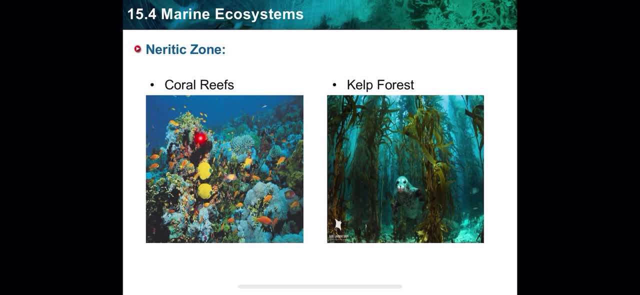 reefs. coral reefs are the most popular coral reefs in the world. coral reefs are the most popular coral reefs in the world areas or in the tropical climatic zone. also in the cold areas or in the temperate climatic zone we can find kelp. look at those green, brown algae brown.